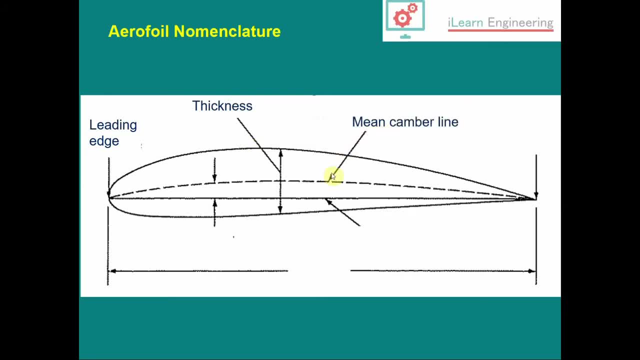 lower surfaces. Here we have a mean camber line, So this is the line that goes from the leading edge to the trailing edge, but it's also equidistant from the upper and the lower surfaces Trailing edge. The chord line is a line that goes from the leading edge to the trailing edge. 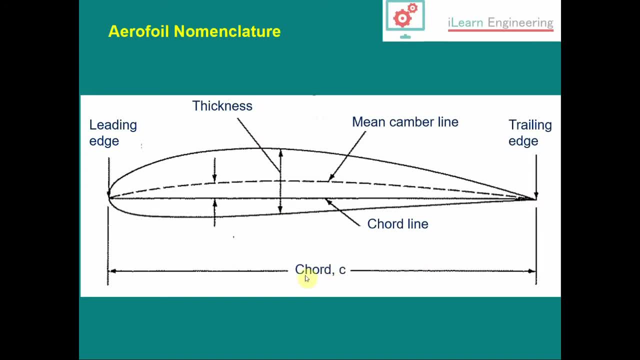 and correspondingly we have a chord length, if you like, which is often has the lowercase c to symbolize it. And finally the camber, which is usually the maximum camber, which is the distance usually measured from the mean camber line to the chord line. 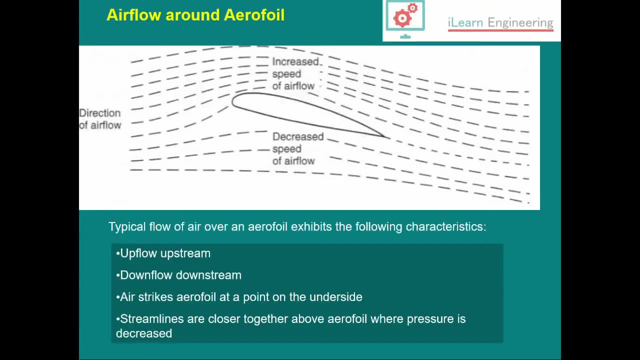 We'll look at some examples later on in the video. Let's have a brief look at the airflow around the aerofoil and, again, the direction of the airflow is left to right and a very simple explanation is one which is often given, which basically goes along. 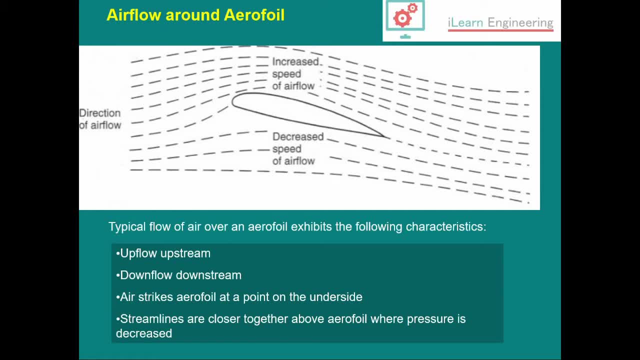 the lines of: well, because the air has to go further over the top than the bottom surface, it has to increase speed. the streamlines, as you can see, get more bunched up and, due to continuity, they go faster Now, and you can then relate Bernoulli's equation to this to obtain some differences in. 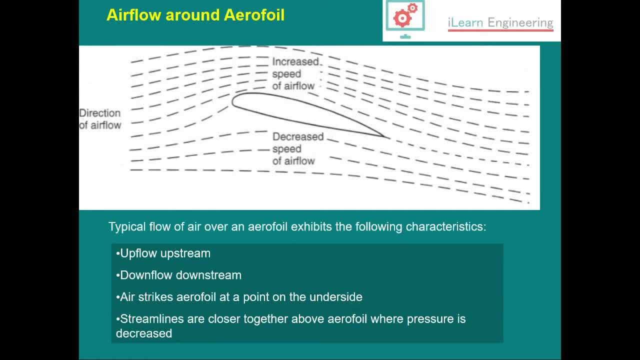 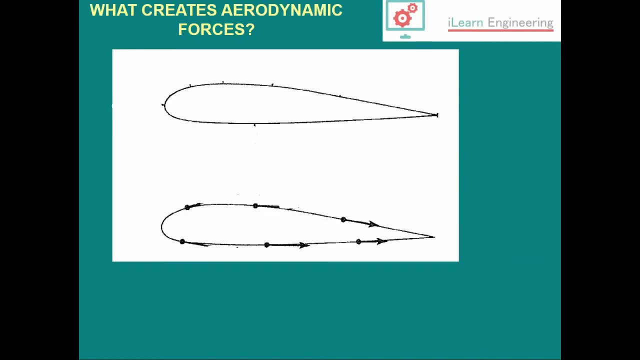 pressure. I'll look on the next slide why there's a slightly different explanation for this. So there's only two fundamental ways in which nature can actually impart the forces onto a aerofoil. So on the top here we have the pressure forces, or the forces due. 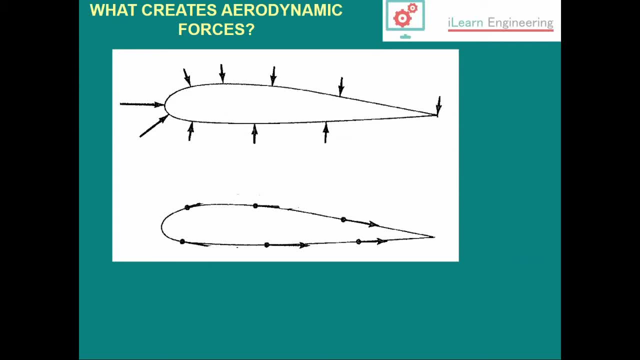 to the pressure. Pressure acts normal to a surface and so, due to the airflow, regardless of what's happening, there's going to be a difference in pressure. So there's a difference in pressure and also going to be a shear force due to the viscosity of the fluid flowing over the object. 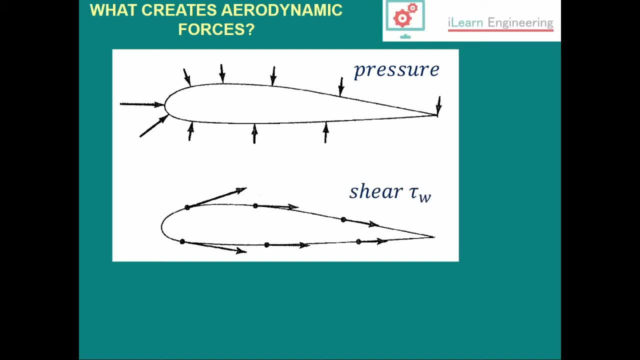 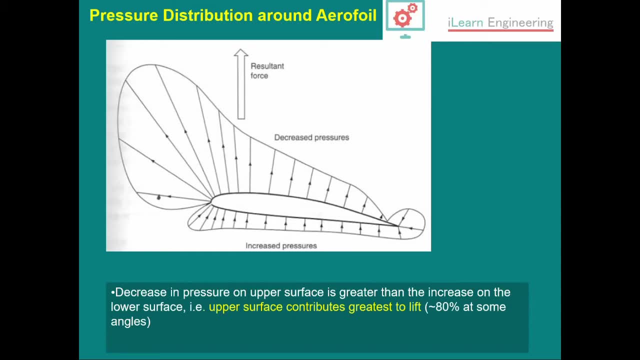 So this is going to result in some skin friction and drag. A slightly better representation of this is given on this diagram and that pressure difference is quite marked and you can see here that the upper surface, which has a decreased pressure and that contributes more to the lift, which is a suction on the top which is pushing. 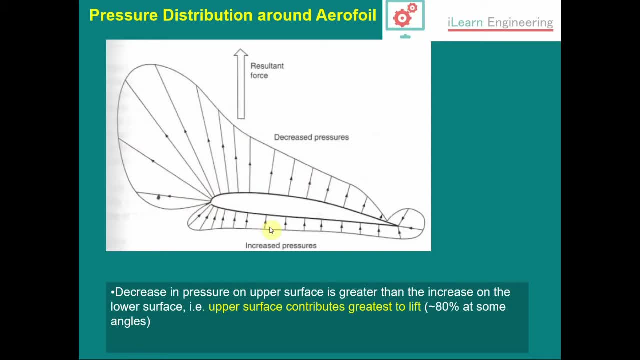 sucking the airfoil up and the increased pressure on the top and bottom surface is pushing it up as well, but that doesn't have as big of an effect as the upper surface. The overall resultant force is: this is some increase. there's a lift force. The main takeaway from this diagram is that it is the 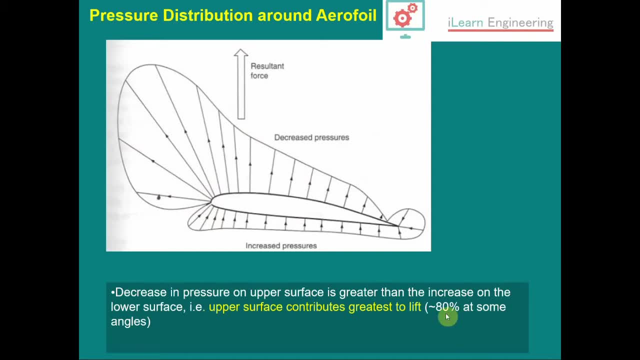 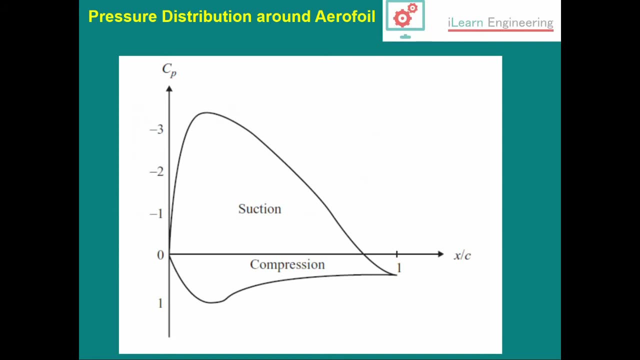 upper surface that contributes greater to the pressure. So the pressure is going to increase to the lift, sometimes as much as 80 percent at some angles. Another way of interpreting that is to look at a plot of the pressure coefficient here. So this is the norm, This is the pressure which has been non-dimensionalized and we will see a very similar 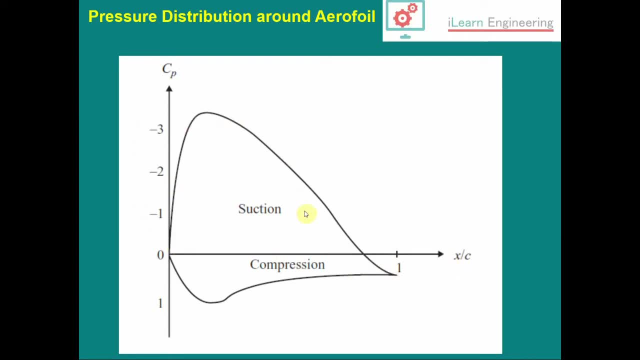 distribution where you can see the negative pressure on the top, corresponding to the suction, and on the lower surface we've got the negative pressure on the top corresponding to the suction. We've got a compression pushing the airfoil up as well, and this is x over c. so this is the distance. 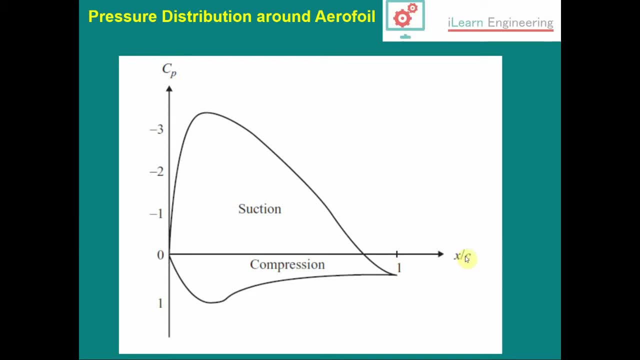 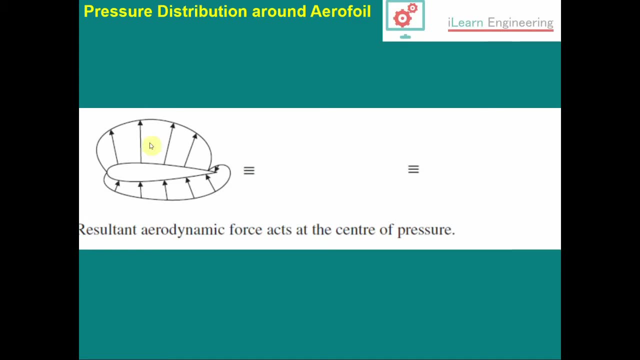 along the chord, The distance along the airfoil normalized with respect to the chord. So this pressure distribution which is shown here on the left, another way of looking at that is that it's equivalent to a single resultant force which acts at one single point, referred to as the center of force. 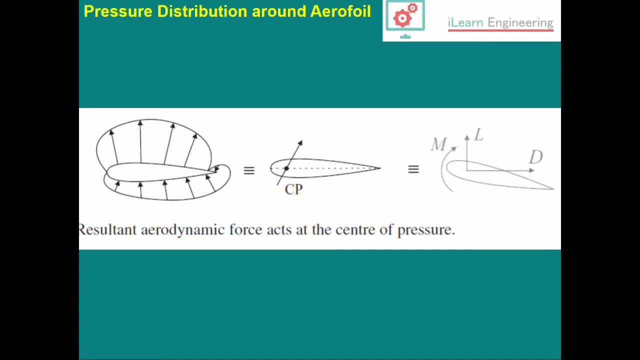 Pressure, and that one single force. well, that can be split into two orthogonal forces and, being right angles to each other, we refer to these as lift and drag, and we would have to put in a moment in there as well to balance it. Looking at that a bit more detail, then we've got a cross section here in the 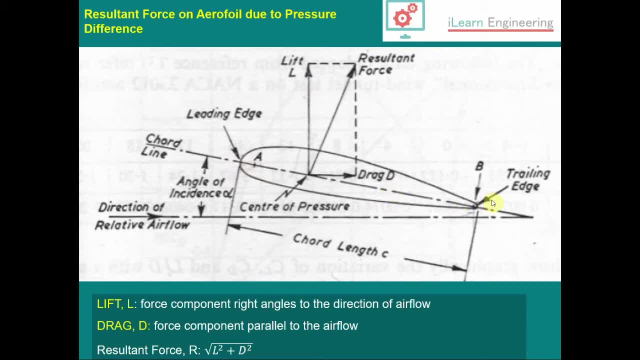 airfoil. We've got the chord line going from the leading gauge to the trailing edge again and we've got the centre of pressure where the resulting force acts due to that pressure differences. and then we resolve that into two perpendicular forces of lift and drag. 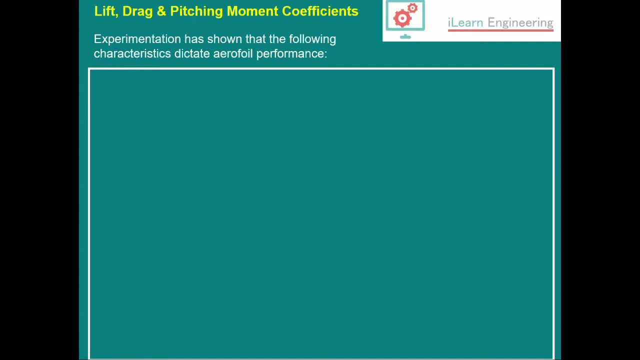 Now it turns out from experimentation that the following characteristics will dictate the aerophone performance: It's the shape of the aerophone, the plan area which we use, the uppercase S for units being metres squared. the square of the velocity, V squared in. 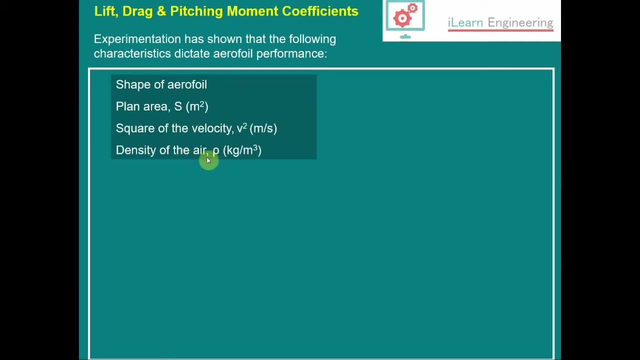 metres per second and the density of the fluid or the air, in this case rho being the symbol. These are the parameters that have been shown to affect these forces, And this results in these common equations, as you've probably seen before, which is that lift equals one. 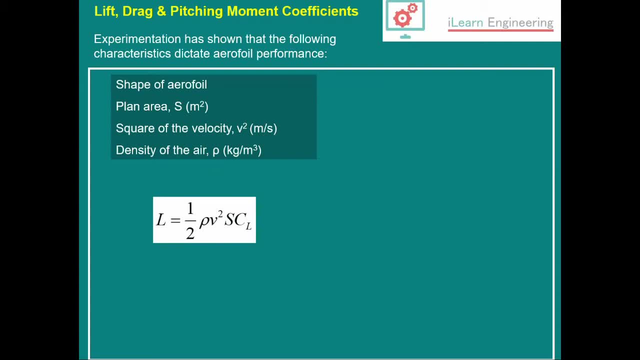 half rho V squared SCL. CL is the lift coefficient. Similarly, for drag we have drag equals one half rho V squared SCD. CD is the drag coefficient and we have an equivalent equation for the pitching moment. So if we take any particular aerophone, we 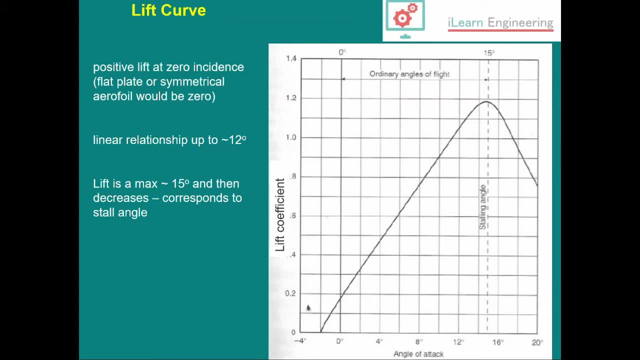 will be able to produce a set of characteristic curves, And one of those is the lift curve, which was shown here. So this is the lift coefficient versus the angle of attack, And what we can see is that we have a linear relationship up to some point here where the lift starts. 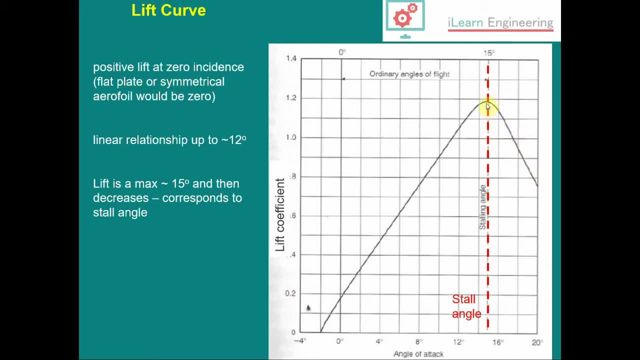 to fall off again. So this is what's referred to as the stalling angle. So, going beyond this, the aerophone goes into what we call a stall. You'll notice that the lift doesn't go to zero completely, but there is a rapid deterioration. 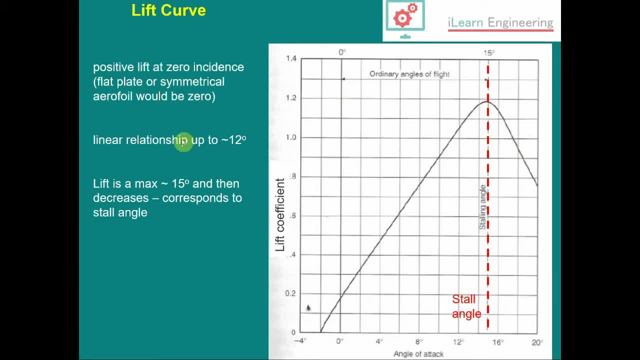 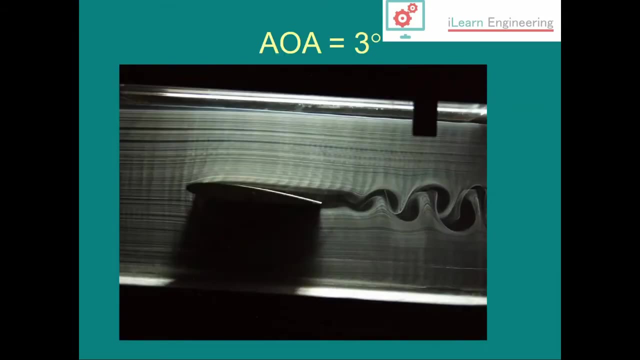 of it. So then, if we want to stay below the stall angle, then you'll see that does help us to define various angles for normal flight to operate within. Here are some pictures from a wind tunnel experiment, something that is called a Stahl angle. This is some real wind. 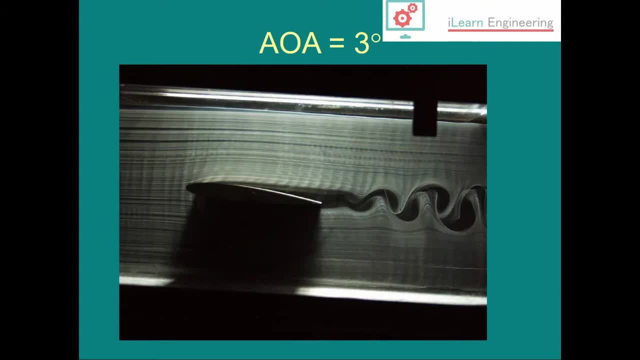 tunnel experiments for aeronautical aeronautics. So I wanna sort of get a feel for what happens between the two angles here. So let's start with the 보면 of the student. but it doesn't aerofoil and you can see there streamlines quite nicely with this flow. 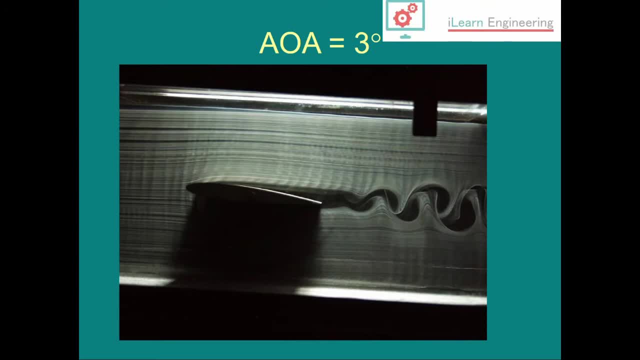 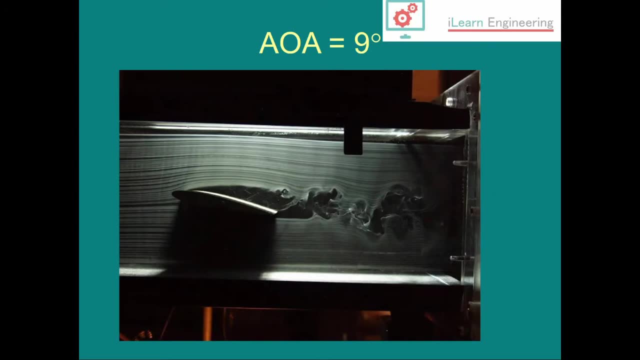 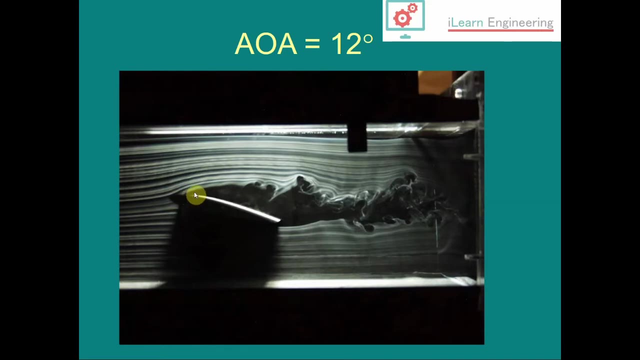 visualization. We've got quite a low angle of attack here of three degrees, and as we increase the angular attack steadily, you'll notice that we start to see a separation of the flow on the upper surface here, so it's starting to go into a stall. Now, if we look at a pictorial representation of what's, 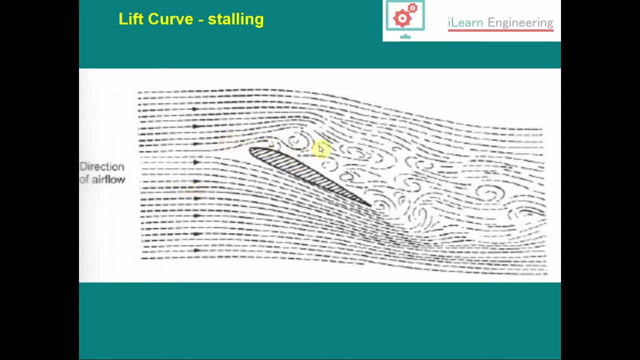 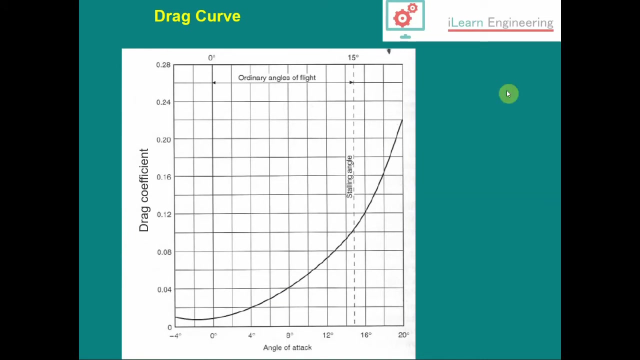 happening at stall and we can see that we get this separation of the flow and it produces a turbulent mixing and it's that which results in a reduction in the lift and an increase in the drag. so you want to avoid this condition. So coming on to drag, then there's another main force for aerofoils. It should come as no. 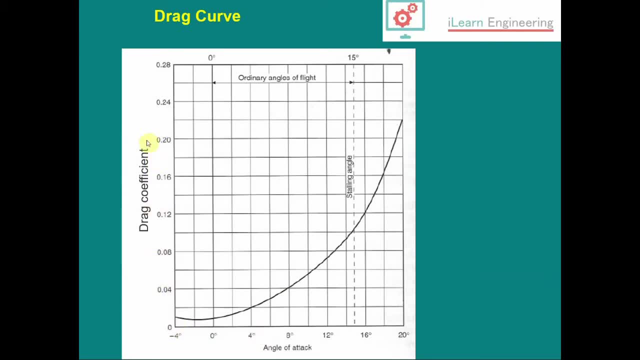 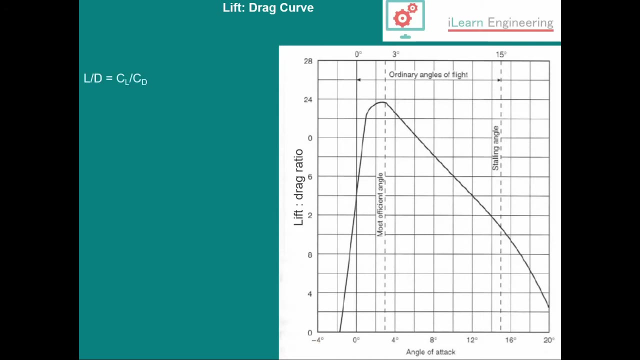 surprise if we've got here the drag coefficient on the axis here and here we've got the Mp of attack. This drag increases as we increase the angle of attack. Now, one thing that we might be interested in is what's known as the lift to drag ratio. 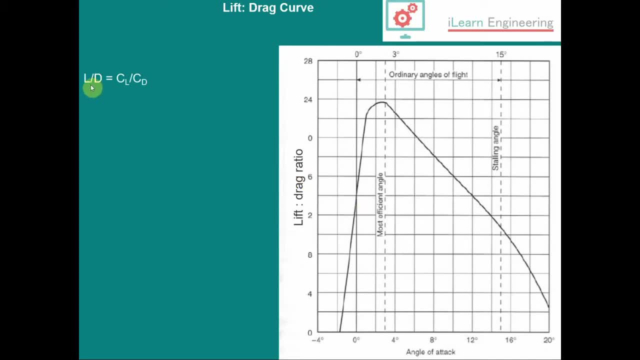 Now on the left, here we've got an equation very simple: lift over drag. Remember that is going to be the same as the lift coefficient divided by the drag coefficient. We want to increase lift and we generally want to decrease drag, and so you can see from this equation if you want to increase the lift and decrease. 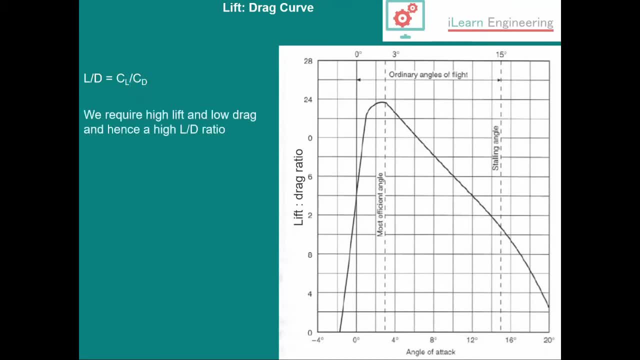 the drag, then the whole ratio of lift to drag is going to be increased. So we're looking for a maximum lift to drag ratio. So if we plot the lift to drag ratio as we've got here on the right, then you can see where it reaches a maximum. that's. 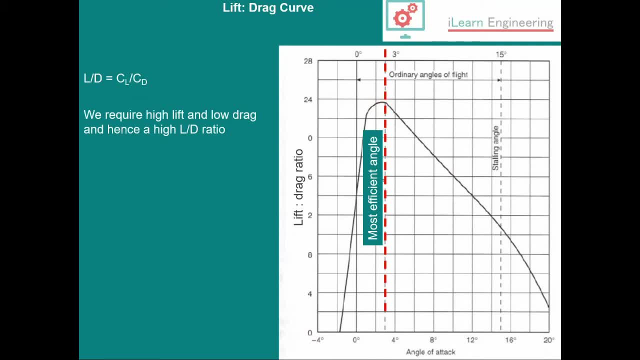 going to be our most efficient angle for the air force to operate at. So these airfoils, if they were fixed at this angle here during the cruise condition, that's going to be our most efficient condition for the majority of the flight, So it's roughly about three degrees for this particular. 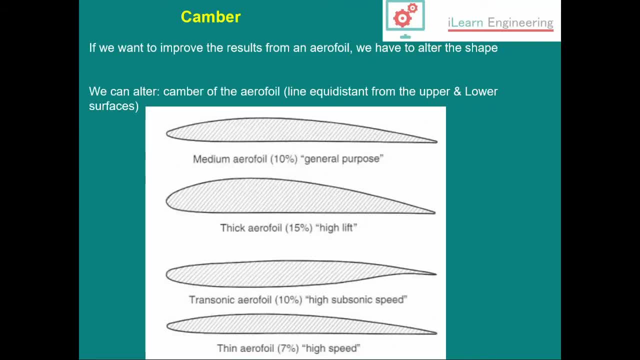 airfoil, for instance. If you want to improve the results for an airfoil, the only thing you can do is alter the shape, and that usually means altering the camber, and that usually means altering the camber, and that usually means altering the camber. 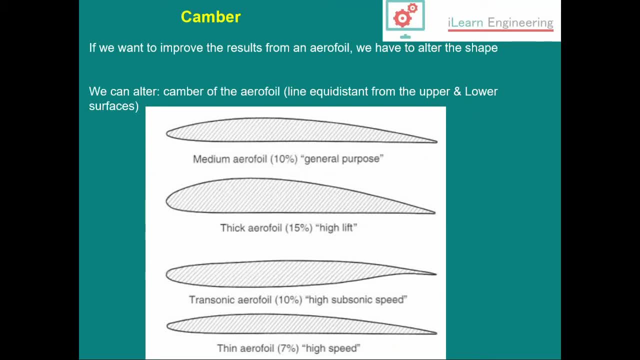 So remember, the camber is the line which is equidistant from the upper and lower surfaces of the airfoil. I've got some examples here. on the screen You can see a general-purpose airfoil. on the top We have a thick airfoil for higher lift. but 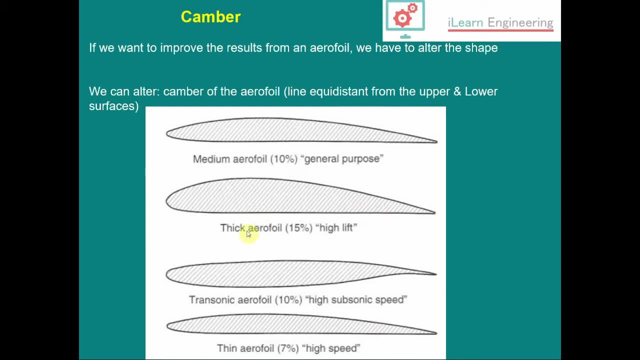 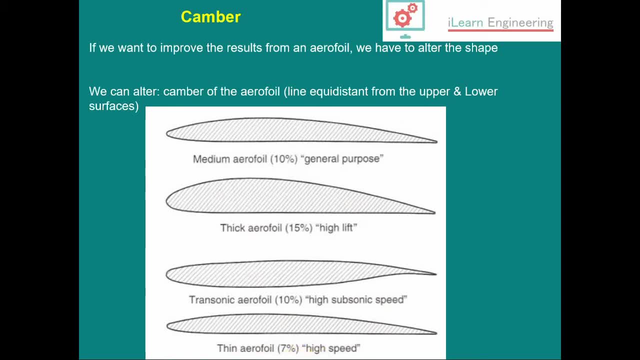 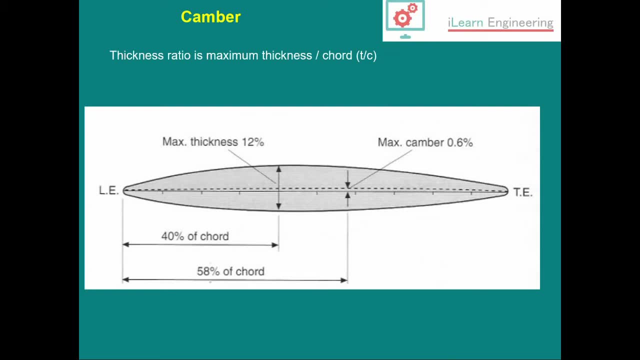 So as you increase your speed you can see that they tend to become thinner. Now we've looked at camber earlier on, but a little bit more detail here. You can see here that the maximum thickness in this example is 12%. I'm sorry, the position of it is at 12% of cord. 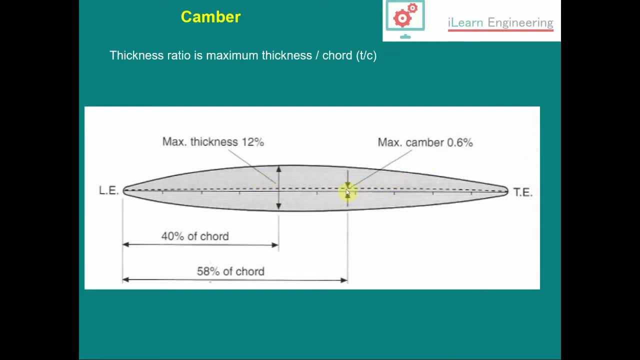 and the maximum camber is 0.6%. So it's not a lot of camber on this particular one, And it happens at 40% of cord for the maximum thickness, whereas the maximum camber happens to occur at 58% of the cord, And these distances are, as quoted, as being downstream of the leaning edge. 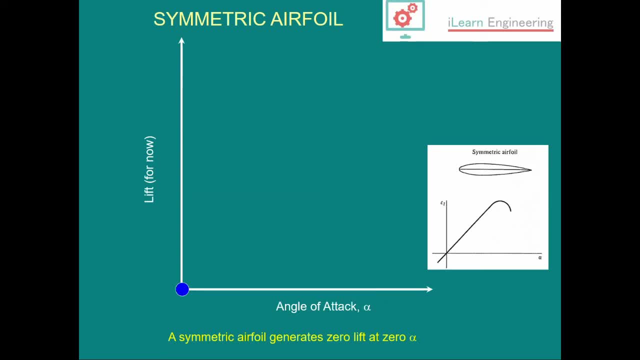 So just in summary, then if we have a symmetrical airfoil, we could use a very simple graph, the linear portion of the lift curve, which is this bit. here it's going to go through the origin of the graph. So in other words, 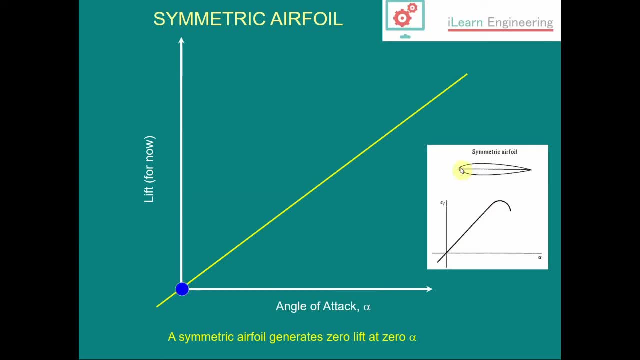 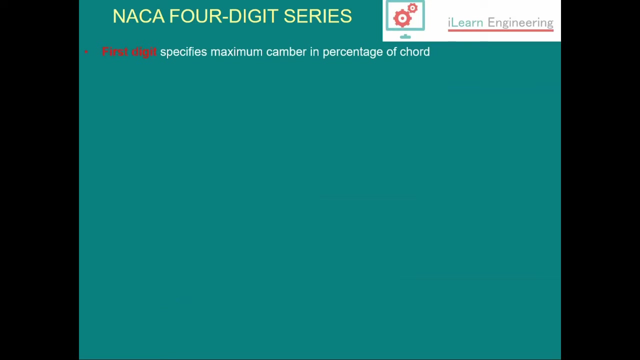 we're not going to produce any lift at zero angle of attack for a symmetrical airfoil. If we move to a camber airfoil, we will notice that we are able to produce positive lift at zero angles of attack. Now, over the years, there are lots and lots of. 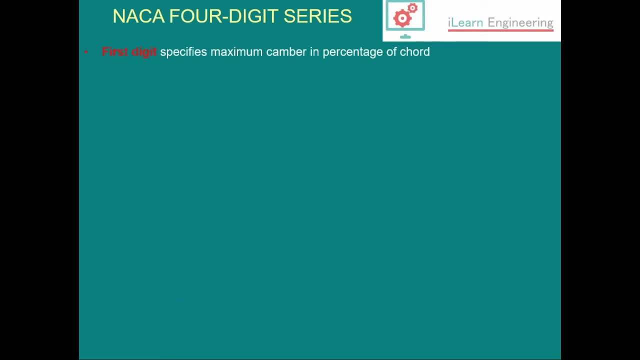 airfoils have been developed and there's lots of families of them. One of the most famous is the NACA series of airfoils and there are four digits and five digit series, et cetera. So I'm just going to look very briefly at a four digit NACA airfoil. 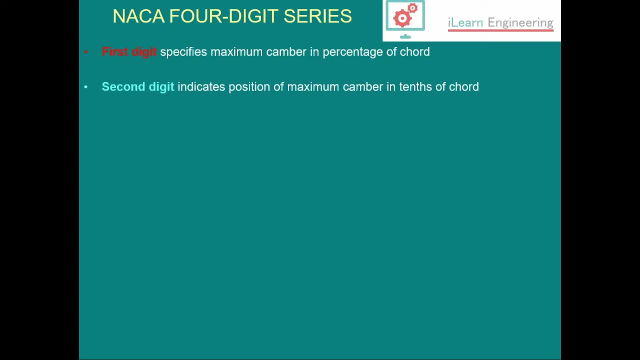 Now, the first digit specifies the maximum camber as a percentage of the cord, whereas the second digit will indicate the position of that maximum camber and it gives that as in tenths As a percentage. and the last two digits they will specify the maximum thickness of the airfoil. 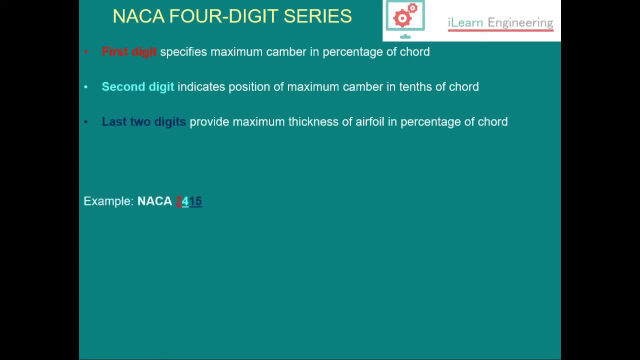 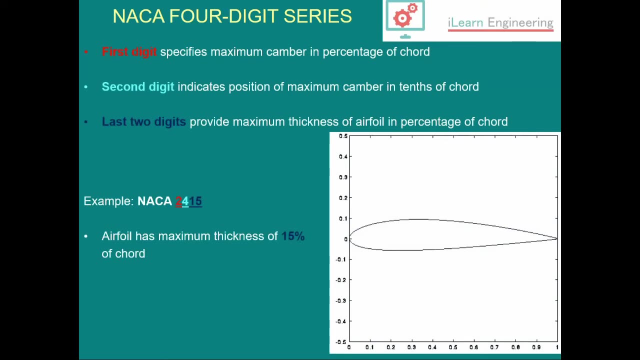 Again, it's a percentage of the cord, Best shown with an example. So I've got the NACA 2415.. So this airfoil is going to have a thickness of 15%, as indicated by the last two digits. This will also have a camber of 2%, as indicated by the first digit, and that will be located. 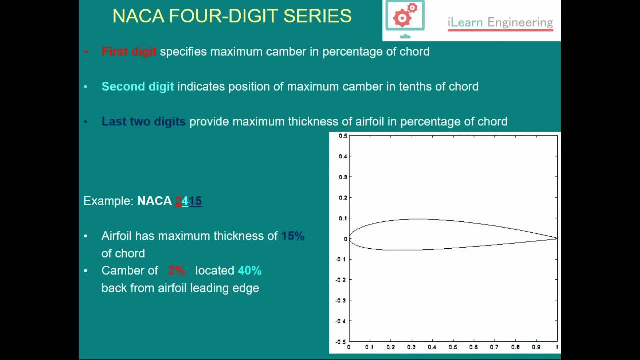 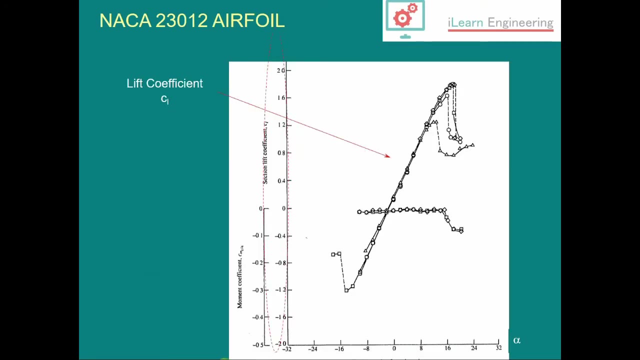 40%, or four tenths of the way back from the airfoil leading edge, as seen here on this diagram. So there are lots of these airfoils that you can find off the shelf, So to speak. I've got another one here which is a 23012, so the five series, This is the set of 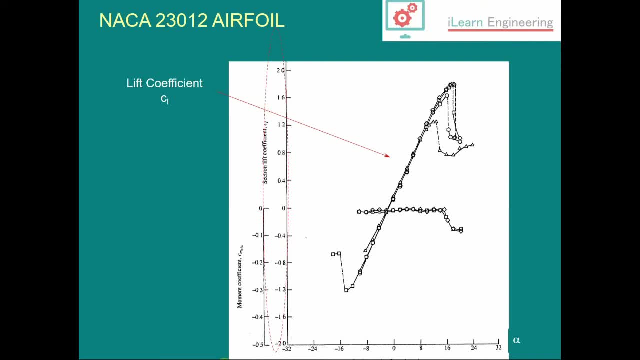 characteristic curves that you can find for airfoils, And you can see that we've got the lift coefficient shown here, which is reasonably linear, And then you will see that we have a stall. Now you can see there's lots of different curves overlaid here. 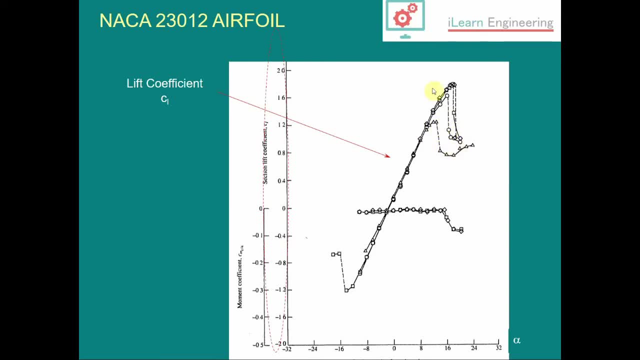 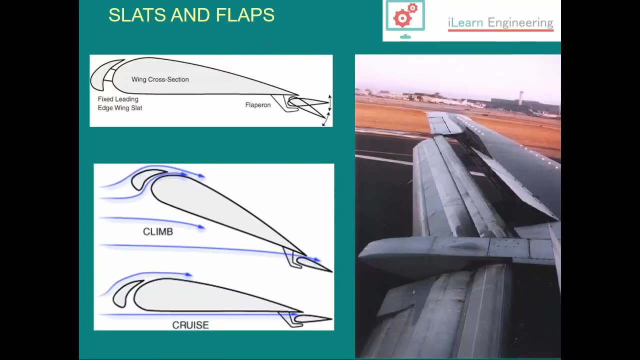 because these are for different Reynolds numbers of speeds, But you can see that within the linear range it's fairly independent of Reynolds numbers. This flat curve here is the coefficient moment coefficient. So one way of delaying a stall is to introduce high lift devices such as slats and 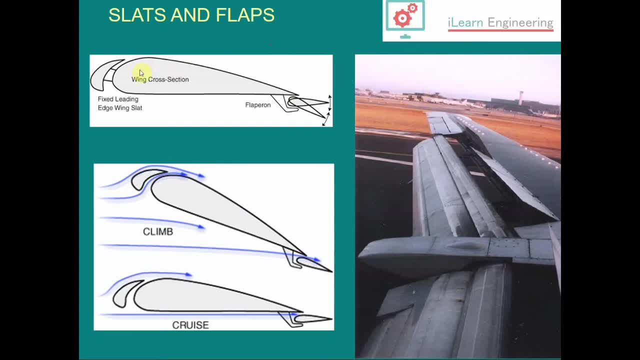 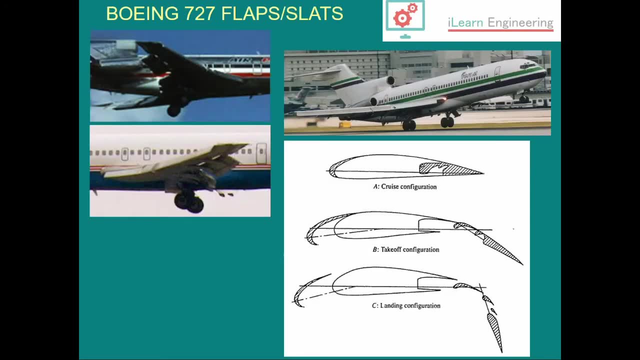 flaps. So we can see on examples of those Boeing 727 for instance. So you'll notice in this cutaway section here that these high-lift devices they're all stowed away during the cruise configuration and then they will clearly they aid to the overall Aerofoil cross. 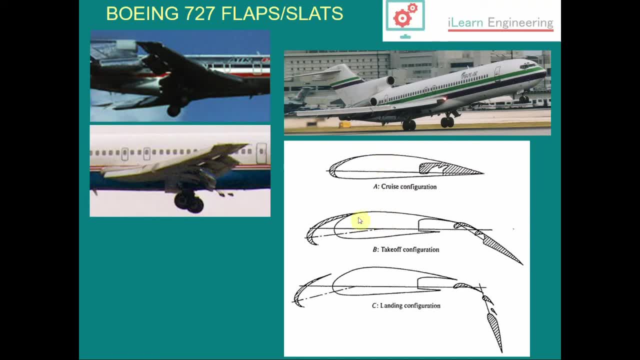 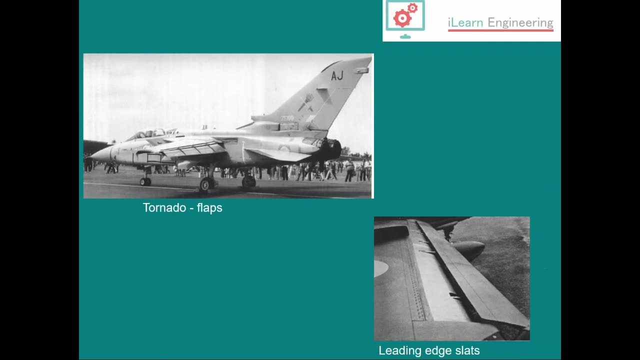 section and then when you need them, they will come out and be deployed and normally there are take-off and landing configurations. You can see the overall camber of the Aerofoil has been increased And a little bit of examples, around the tornado, for instance. Again, if we take a 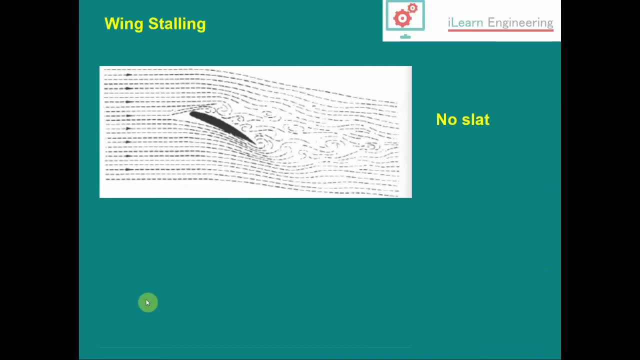 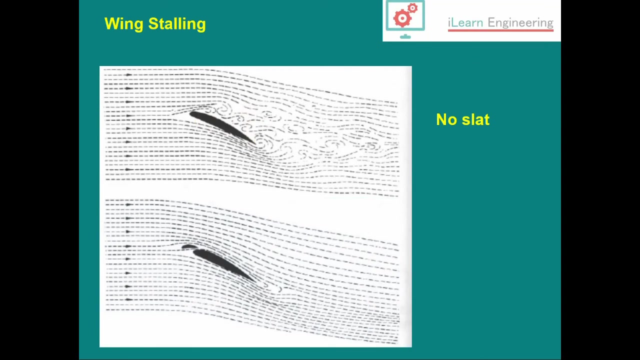 snapshot of the streamlines during a storm. then, as we've shown before, without a slat, just a slat, a basic Aerofoil here, then we get the flow separation on the upper surface and that leads to this loss in lift and an increase in drag. And if we incorporate 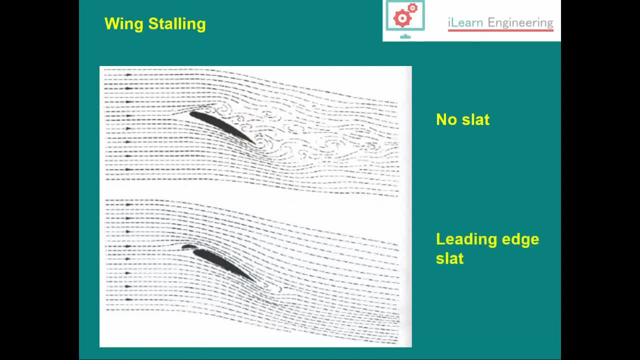 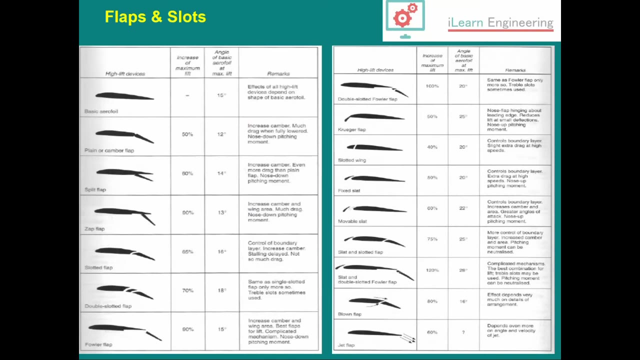 for instance, a leading edge slat, then that helps to delay that flow separation on the upper surface and therefore we're able to maintain the lift and reduce the drag. Lots of high-lift devices are available and you will find them yourself when you do your research. 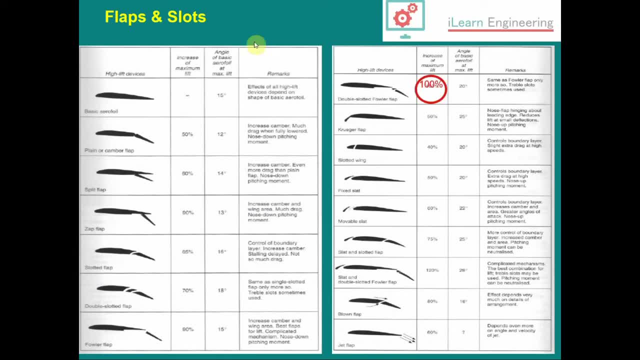 I've given you some examples here. it's not very clear, but on the top left here we've got the basic Aerofoil and there are lots of different examples of how you can increase the lift coefficient. Interestingly, what I've put on here is this double slotted Fowler flap system, because the increase in maximum lift is 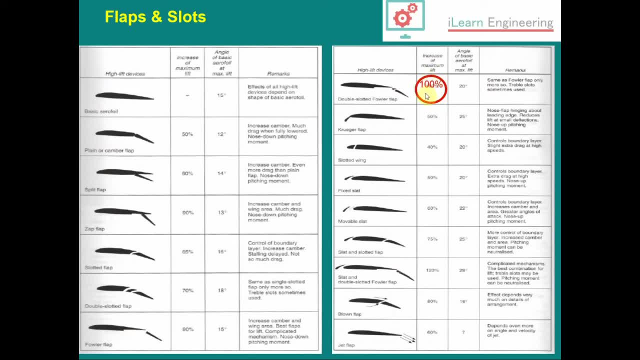 a hundred percent, so it doubles the lift available to you. It's quite quite formidable really. so you can get quite a good increase in performance. Clearly, you're going to get an increase in drag as well, so you're not going to want to use this. 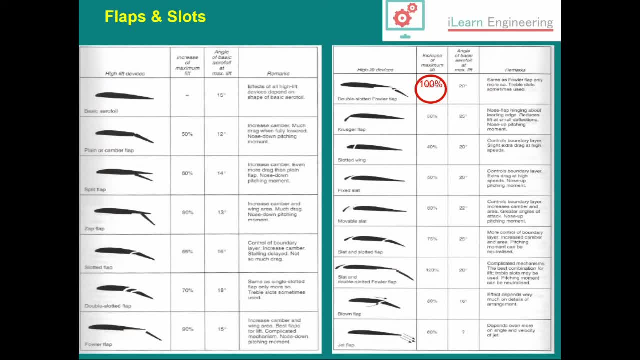 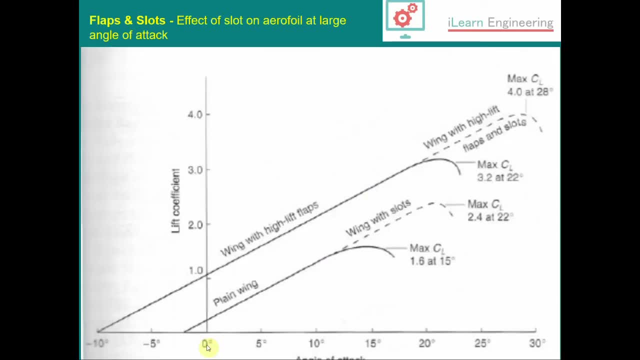 all the time you're going to want to use it when you really need it, at low speeds, which will take off and landing. So this graph is quite interesting because it shows on the bottom here for the plain wing, and then as you increase that wing with high lift flaps we get to the whole graph basically shifts upwards. 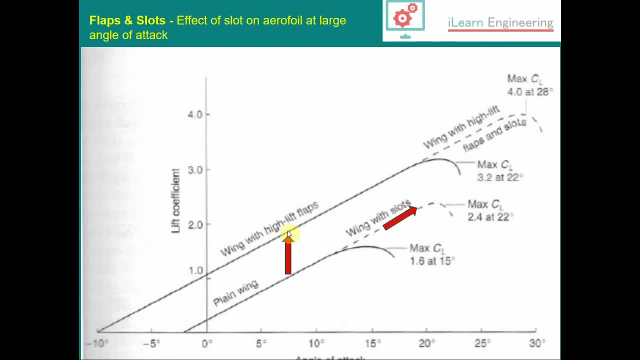 because we've increased the overall camber. It's interesting when we add the slots as well, we're able to increase the drag that we're getting from the top left increase in this direction. So when you increase, you want to introduce both. 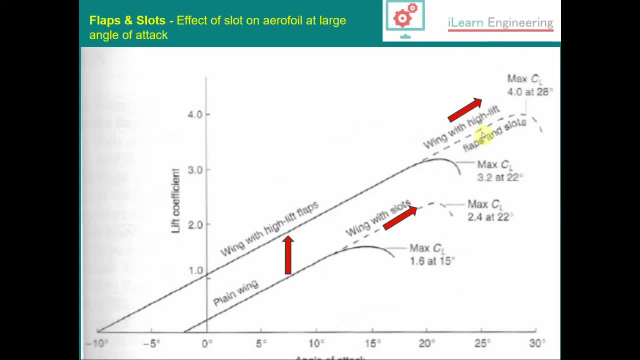 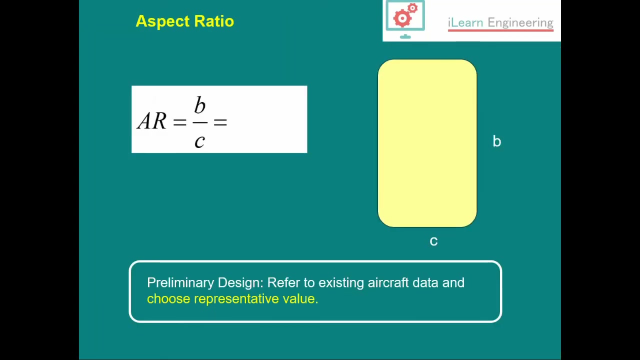 flaps and slots, then you make quite a significant increase to your lift coefficient. So you can certainly get your extra lift, but always remember it's going to be associated with an increase in drag, so it's available for when you need it. So very briefly then, just at the end, and we've looked just at our 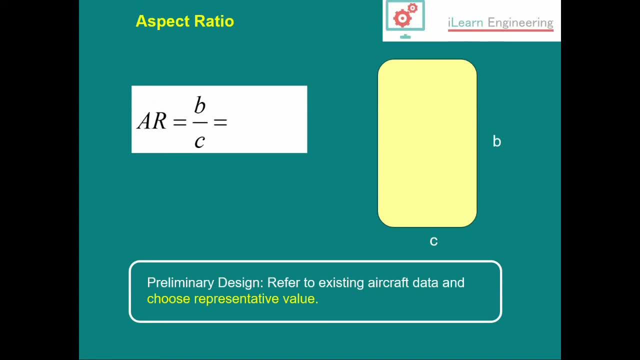 funnels in this brief presentation so far, which is the cross section of the wing. I'm now taking a plan view and when we do that, one of the characteristic features we're looking at is the aspect ratio and just very simple definition. here We take. 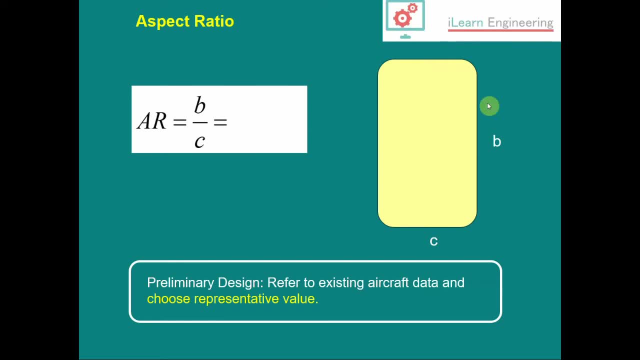 this rectangle and the aspect ratio is the wing span, if you like, divided by the chord C. so you'll be able to see: if you multiply top and bottom of that equation by B, then you will get b squared on the top and you will get bc on the bottom, and bc is the area which we know as s. 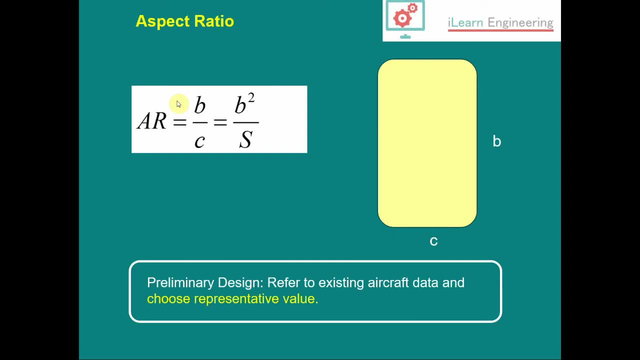 so that's another way of formulating that equation. the key here for obtaining the values of aspect ratios for your preliminary aircraft design is to refer to existing aircraft data and choose a representative value, just as we did in our similar video earlier on. if you look at 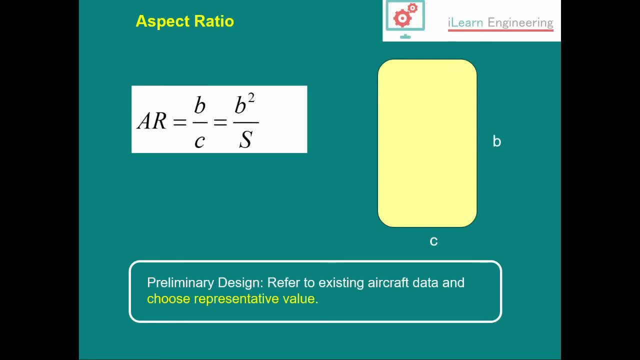 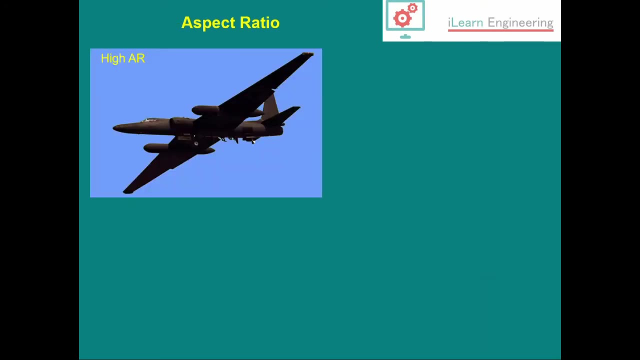 our earlier videos for wing loading and thrust loading from island engineering. you'll notice that we did something very similar there. we tabulated the values for wing loading and thrust loading, and you will see that there are various patterns, and so it is not unreasonable for you to take a representative value. just a quick example of what high aspect ratio and 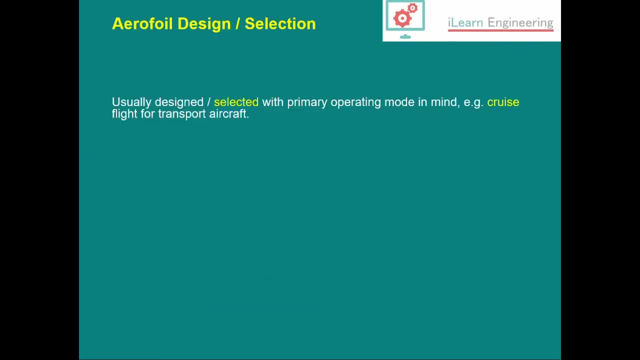 low aspect ratio aircraft look like. so, when you are designing your aircraft and you want to select an airfoil, what you're going to be thinking about is selecting it with the primary operating mode in mind, which is, for example, cruise for a transport aircraft, and then you want to introduce 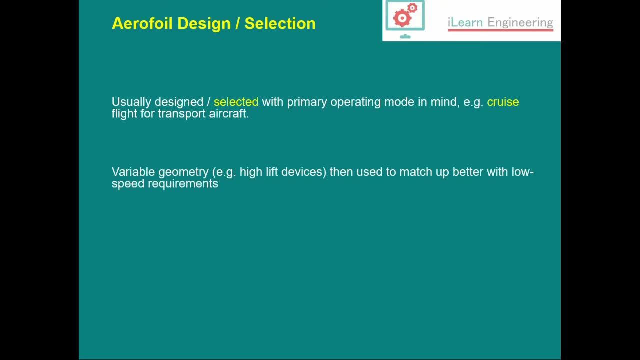 these variable geometry, ie high lift devices, so that you can get your extra lift for your low speed requirements at landing and takeoff. you can select an existing airfoil from the thousands that for you. you don't need to reinvent the wheel. so for your final wing design, having chosen your 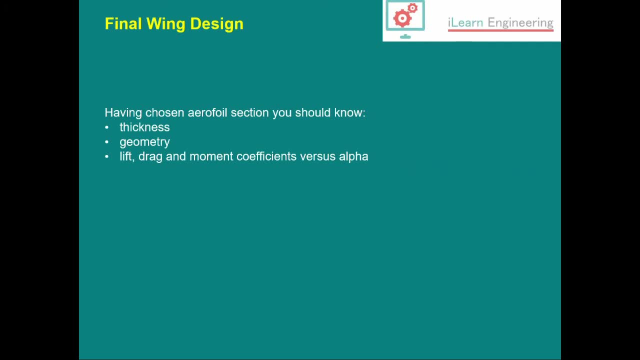 airfoil selection. you should now know the thickness, the geometry, the lift and the drag and the moment coefficients versus your angle of attack, because all of those characteristic graphs will already have been produced and they will be available with the airfoil data you need to decide on. 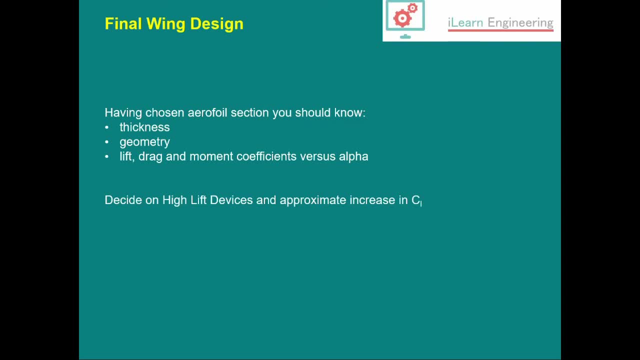 higher lift devices by selecting an approximate increase in lift coefficient. you can choose a representative value for your aspect ratio by looking at existing aircraft designs and, given that you know your wing area s by looking at wing loading, for instance, from an early video, it then becomes possible for you to then calculate the wingspan and the chord, so you